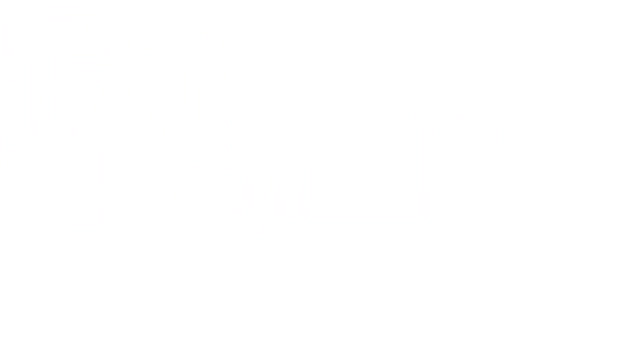 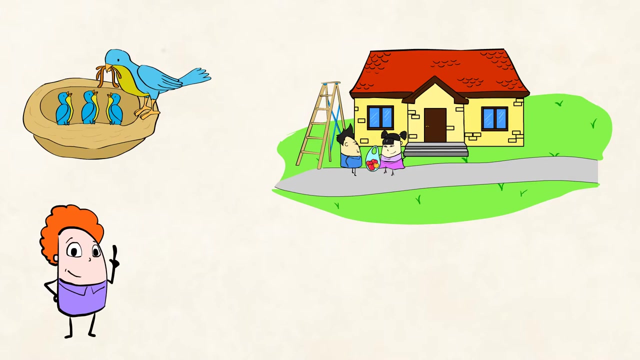 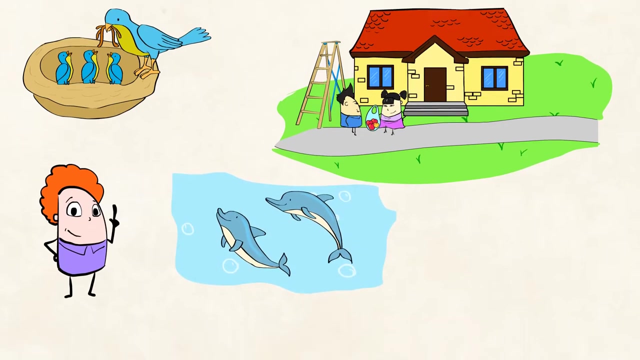 Hello, this is Mighty Owl. We, just like other animals in the animal kingdom, spend our time making sure we have enough food and shelter for ourselves and our families. We also find some time to rest and have fun, though, right, We go on road trips, fly to other countries or go camping in the woods. 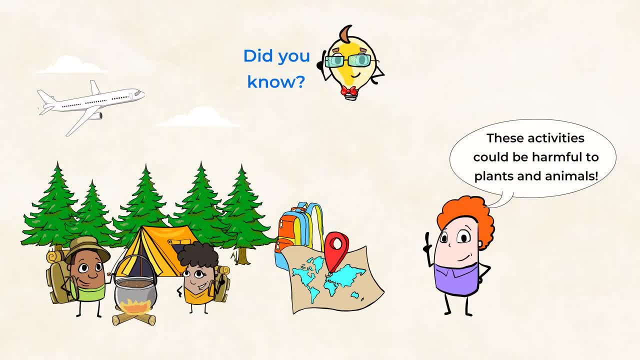 Did you know that all these activities could be harmful, though, to plants and animals? What, No, no, no. It is important to understand how our seemingly harmless activities can affect the environment. Now you may ask: what is an environment? 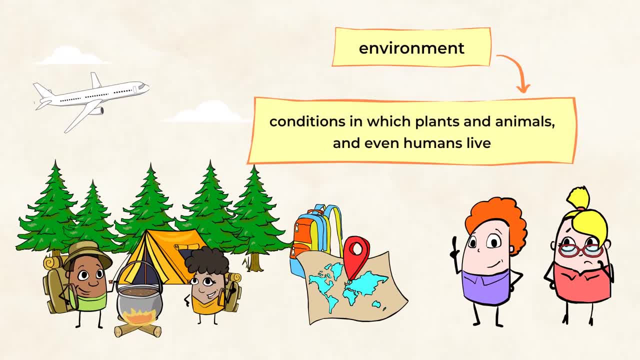 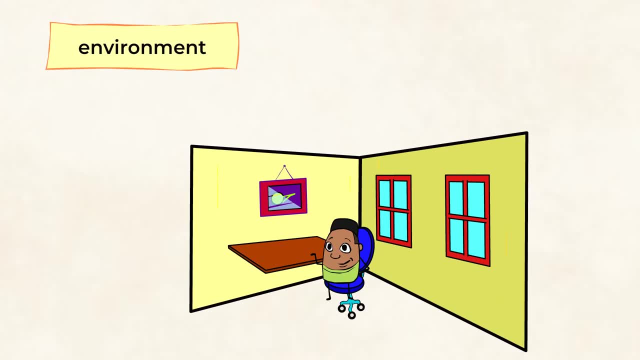 Well, I'll tell you. It is certain conditions in which plants and animals, and even humans, live. Look around you. Maybe you're sitting on a chair in your room, in your house, on the street, where you skateboard with your friend in your town. 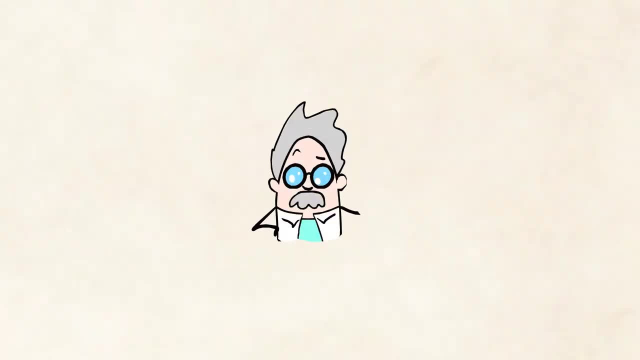 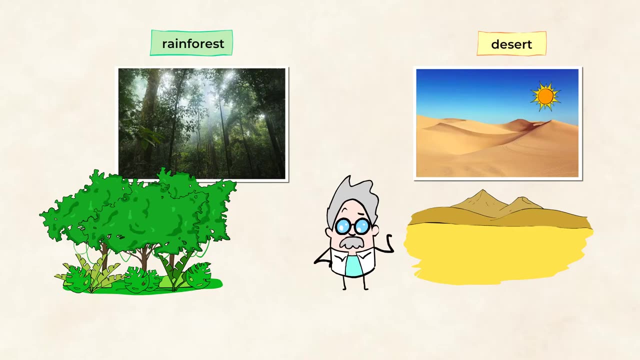 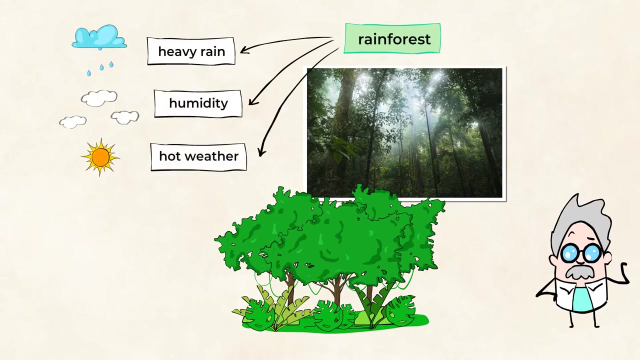 This is your environment, But let's take a closer look at some different environments, like a rainforest or a desert. They're both very different, right? A rainforest is characterized by heavy rain, humidity and hot weather. Can you think of some of the animals that live there? 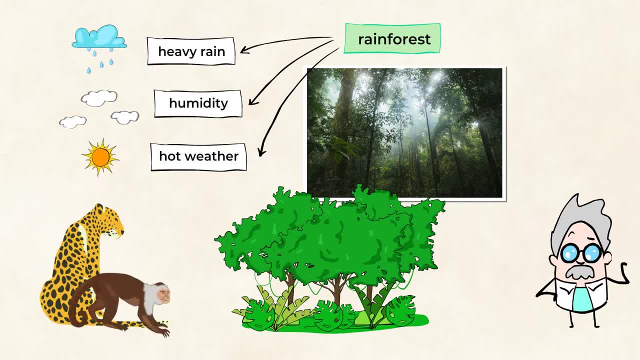 That's right. Jaguars, monkeys, different kinds of birds, snakes and many other kinds of animals. The common feature among them, however, is that they all adapted to living in that specific environment, with plenty of lush vegetation, rainfall and humidity. 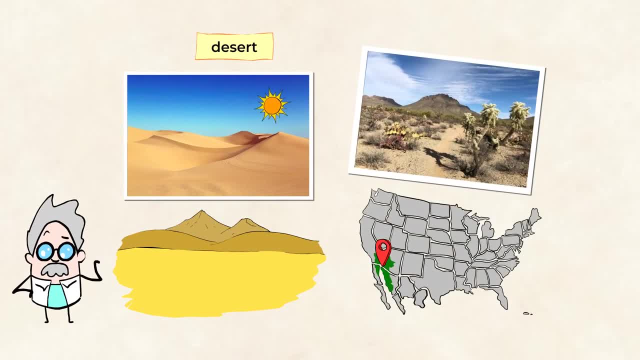 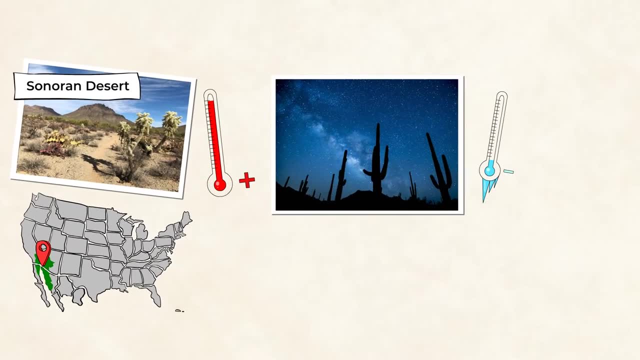 On the other side of the spectrum you have deserts, For example the Sonoran Desert, where temperatures vary from very hot during the day to really cold at night, with very little rain. Do you know that a week of rainfall in a rainforest equals that of a year in the desert? 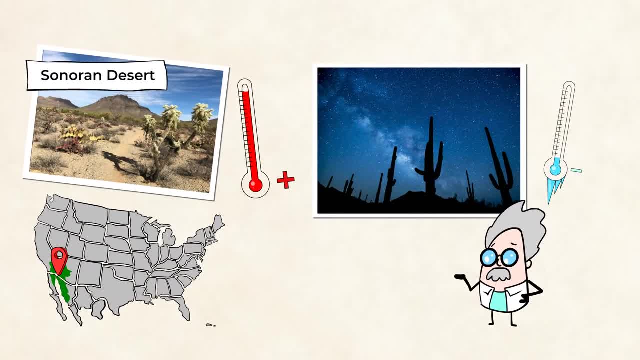 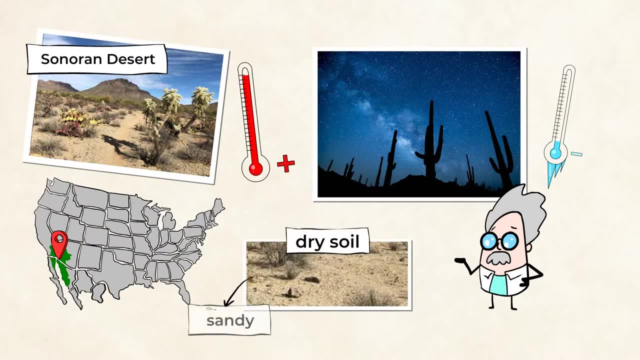 Crazy, right. What else can you think of as a characteristic for a desert? If you were thinking dry soil, that is exactly right. Soil in the desert is sandy and rocky, with few nutrients. That's why vegetation is very different in a desert. 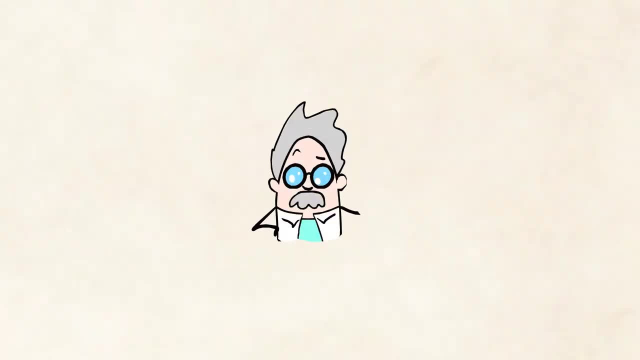 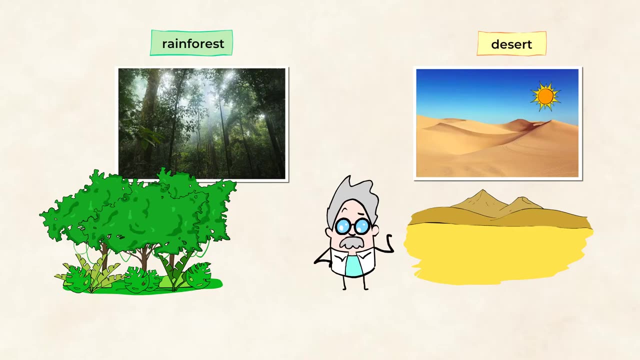 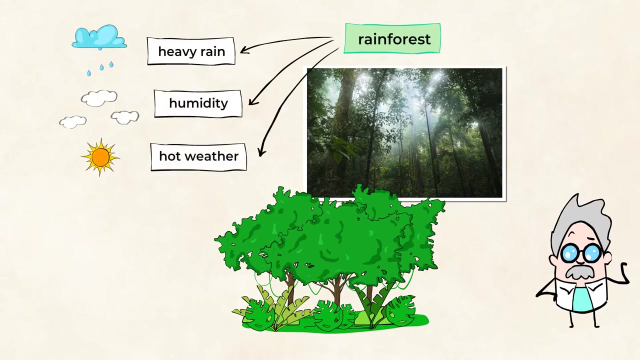 This is your environment, But let's take a closer look at some different environments, like a rainforest or a desert. They're both very different, right? A rainforest is characterized by heavy rain, humidity and hot weather. Can you think of some of the animals that live there? 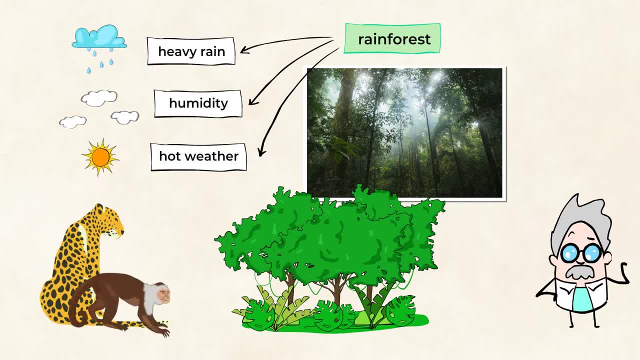 That's right. Jaguars, monkeys, different kinds of birds, snakes and many other kinds of animals. The common feature among them, however, is that they all adapted to living in that specific environment, with plenty of lush vegetation, rainfall and humidity. 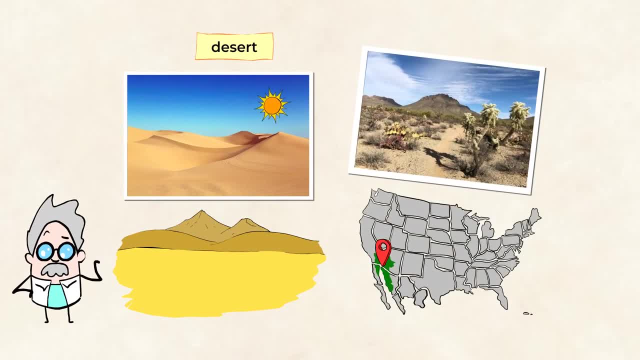 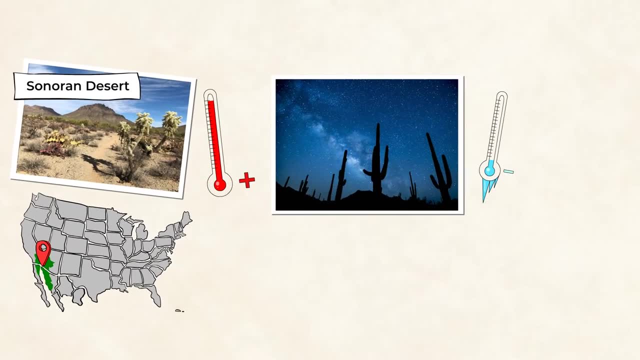 On the other side of the spectrum you have deserts, For example the Sonoran Desert, where temperatures vary from very hot during the day to really cold at night, with very little rain. Do you know that a week of rainfall in a rainforest equals that of a year in the desert? 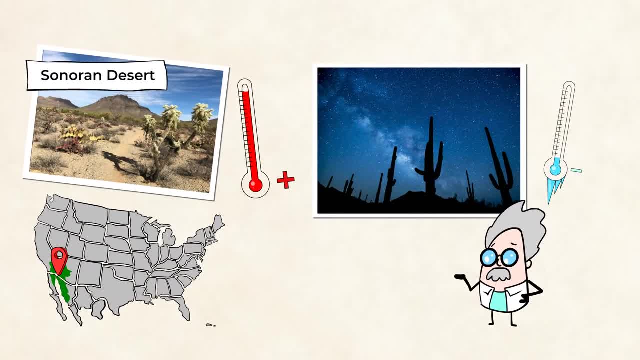 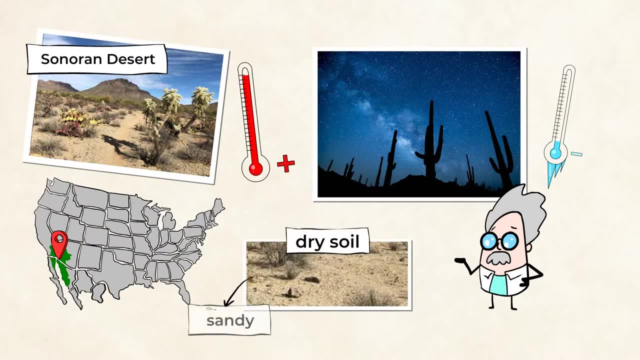 Crazy, right. What else can you think of as a characteristic for a desert? If you were thinking dry soil, that is exactly right. Soil in the desert is sandy and rocky, with few nutrients. That's why vegetation is very different in a desert. 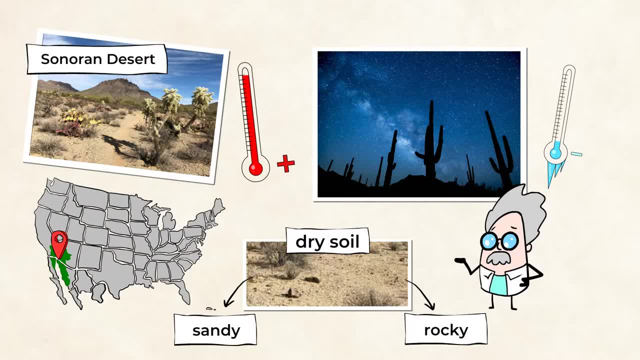 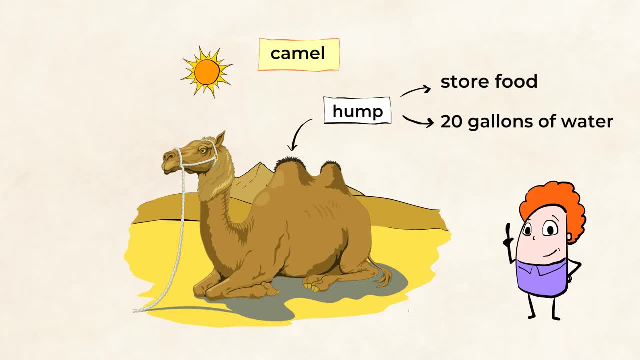 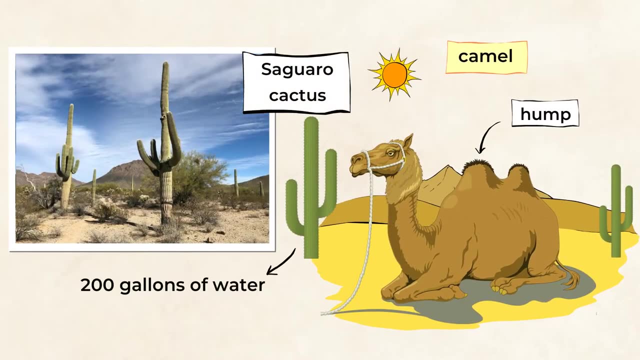 Animals and plants have adapted to living in long periods of time without any water. A camel has a hump to store food and can drink up to 20 gallons of water at a time. Cacti can store water for even longer periods. A saguaro cactus can soak up to 200 gallons of water during a good rainfall. 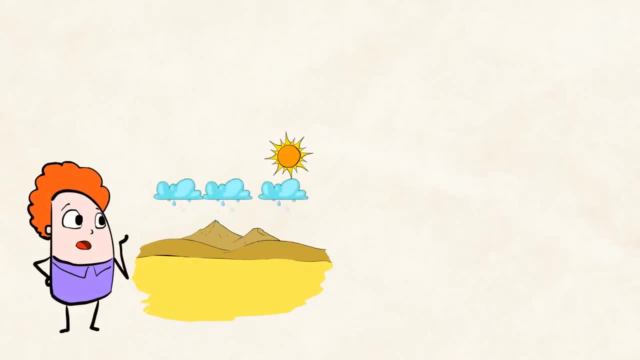 But what do you think will happen if, all of a sudden, there is more rain in the desert Or less rain in the rainforest, Or if we chop down trees in the rainforest Or even burn the trees? You know what will happen. 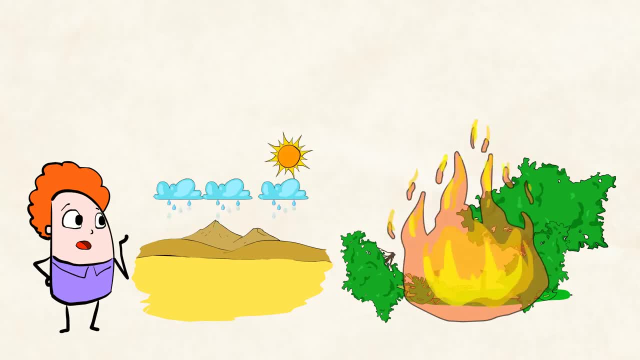 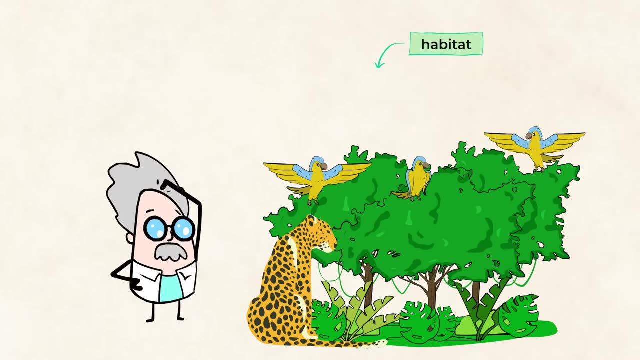 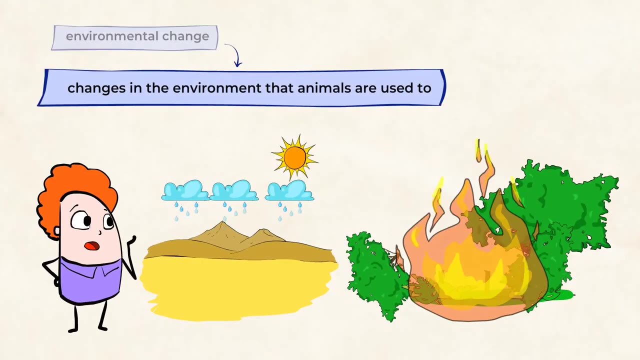 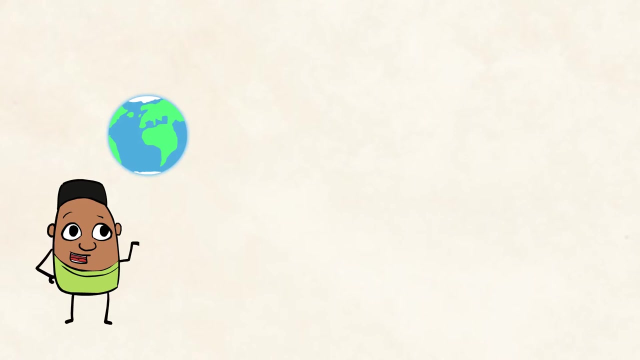 The living conditions will change. All these will upset the delicate balance of the food chains in their respective habitats. A quick reminder: A habitat is where an animal lives. Such changes in the environment that animals are used to are called environmental change. Many, many years ago, the earth looked a lot different from what it looks like now. 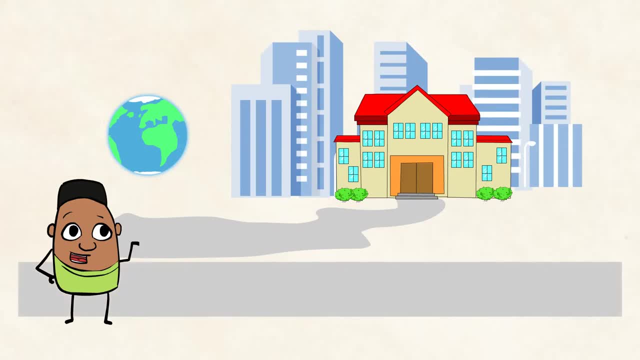 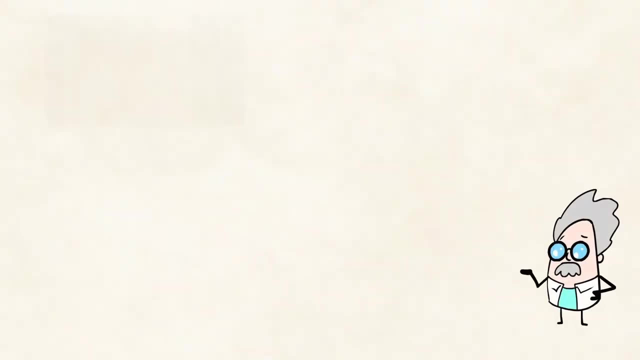 No matter where you lived- in a big city or a town or a small village- there were no roads, schools or buildings back then. Most likely there was wilderness, such as forests, wetlands, grasslands and beaches. 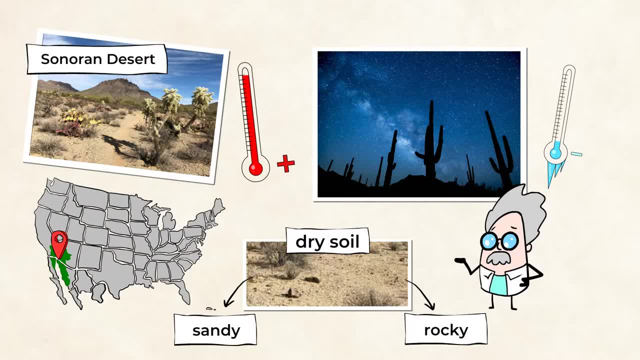 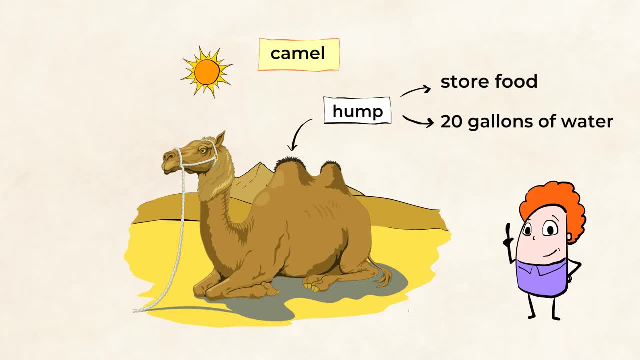 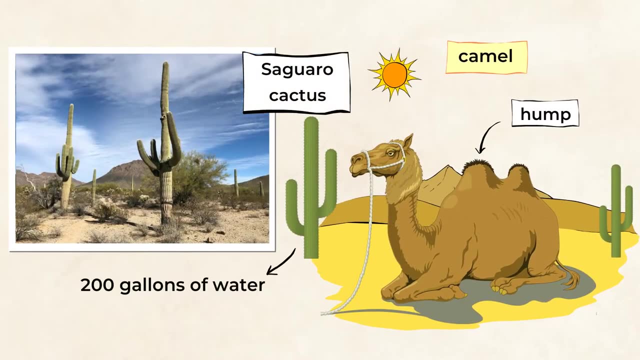 Animals and plants have adapted to living in long periods of time without any water. A camel has a hump to store food and can drink up to 20 gallons of water at a time. Cacti can store water for even longer periods. A saguaro cactus can soak up to 200 gallons of water during a good rainfall. 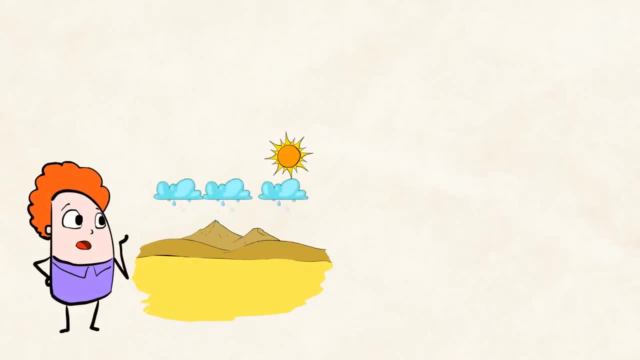 But what do you think will happen if, all of a sudden, there is more rain in the desert Or less rain in the rainforest, Or if we chop down trees in the rainforest Or even burn the trees? You know what will happen. 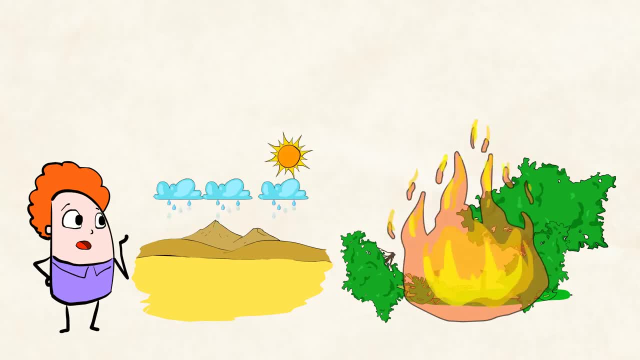 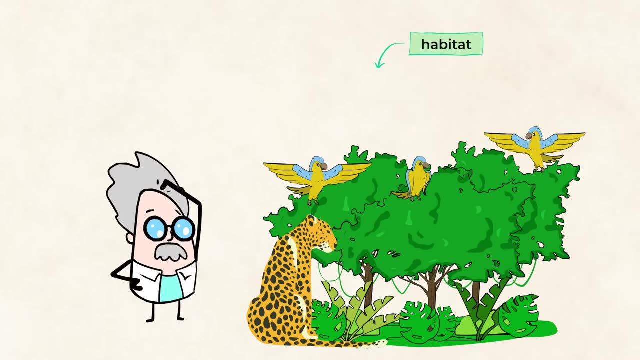 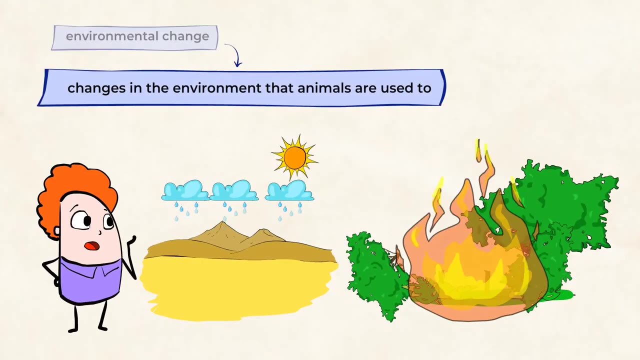 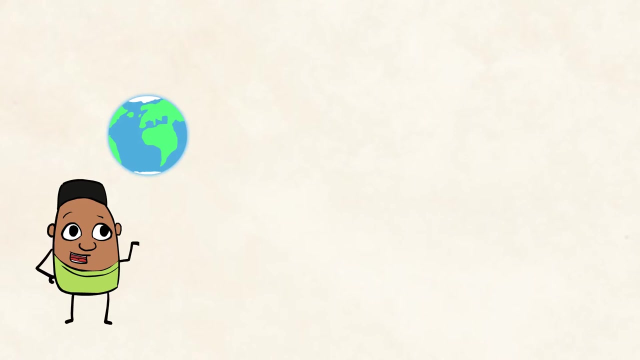 The living conditions will change. All these will upset the delicate balance of the food chains in their respective habitats. A quick reminder: A habitat is where an animal lives. Such changes in the environment that animals are used to are called environmental change. Many, many years ago, the earth looked a lot different from what it looks like now. 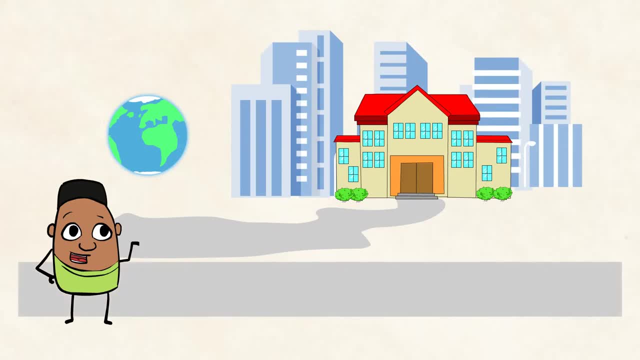 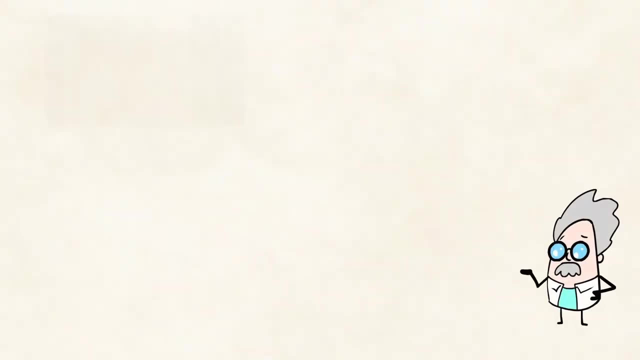 No matter where you lived- in a big city or a town or a small village- there were no roads, schools or buildings back then. Most likely there was wilderness, such as forests, wetlands, grasslands and beaches. 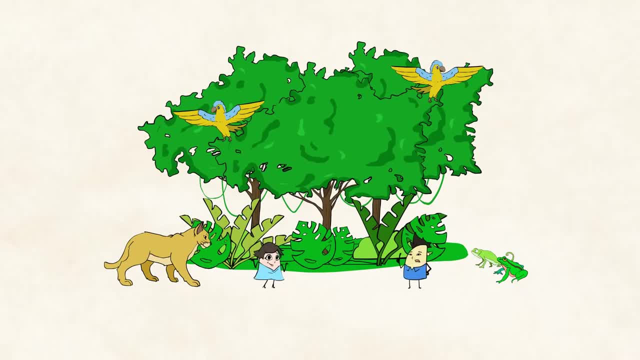 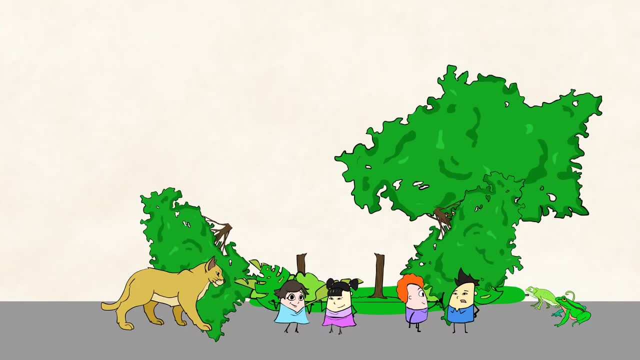 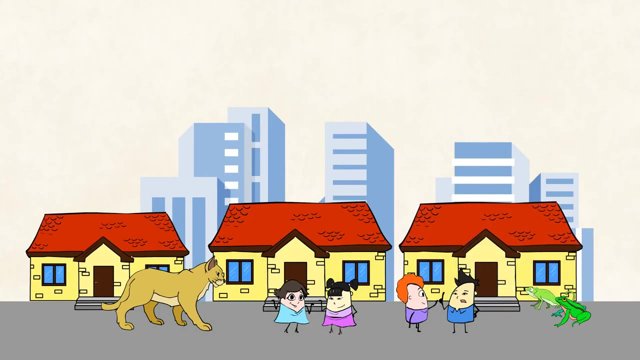 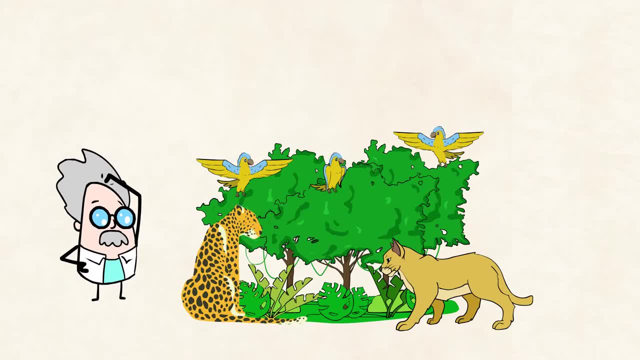 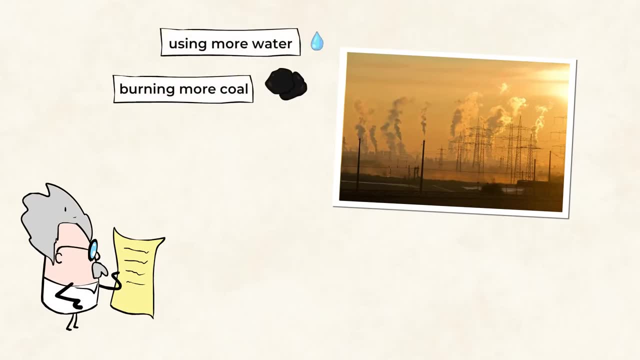 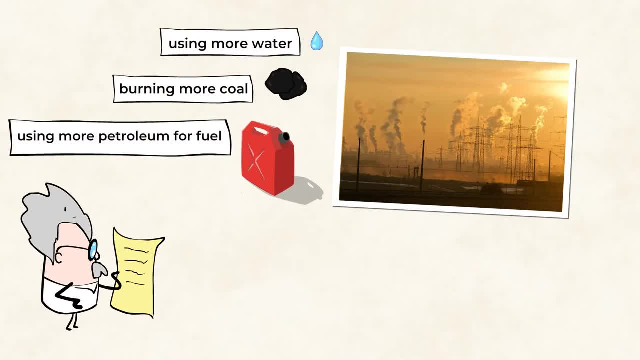 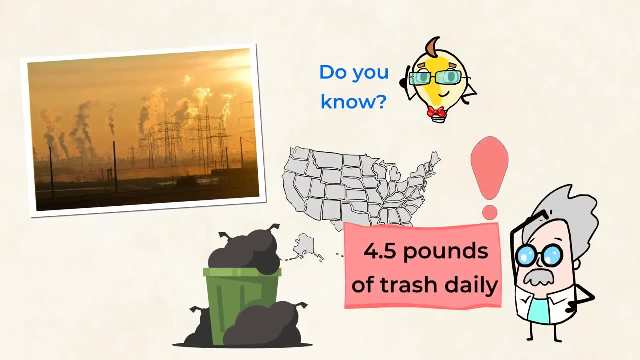 And the more we use them, the more bad chemicals are released and the more garbage is generated. Do you know that a person in the United States creates 4.5 pounds of trash a day? That's an enormous amount. Cars, buses and cars. 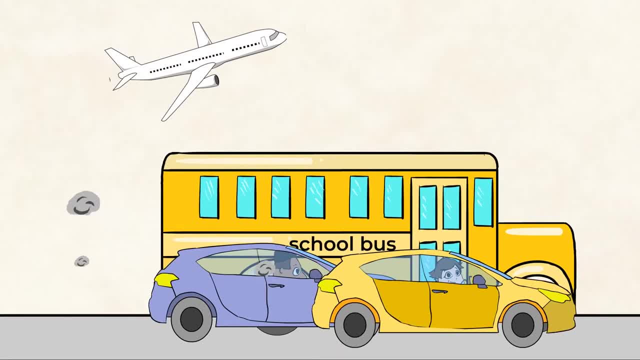 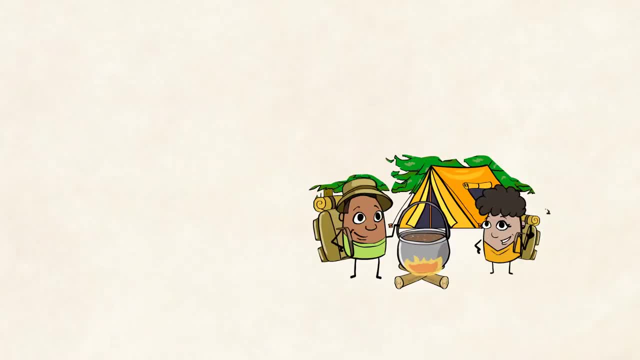 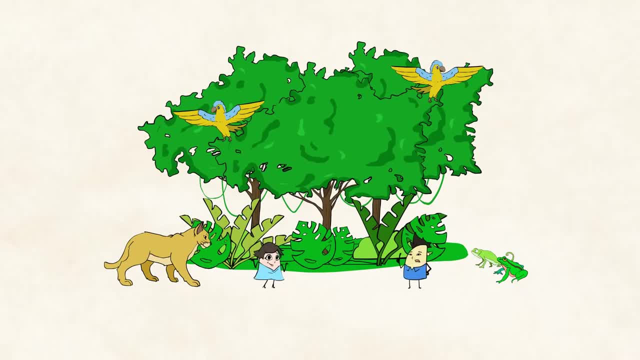 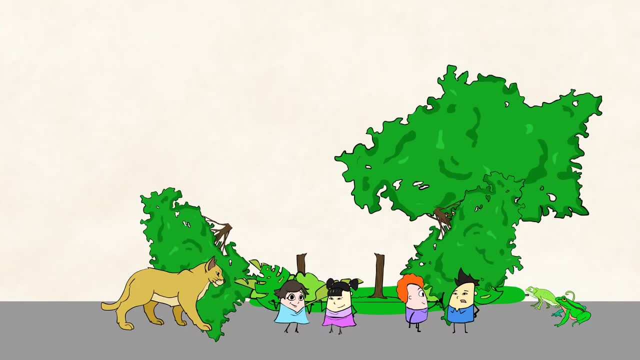 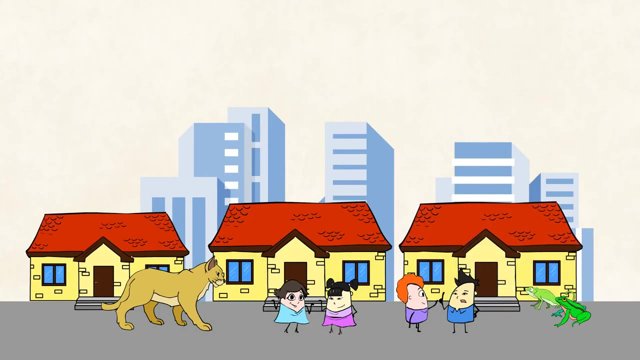 But over time, as the human population grew and evolved, we had to create our own habitat, So we carved out roads into the landscape, chopped down trees and built factories. These environmental changes affected the ranges of animals and plants in those areas. 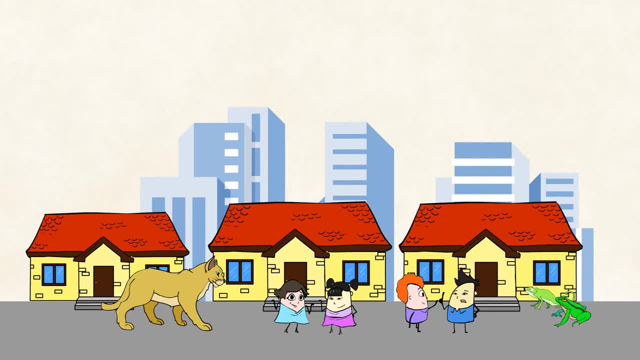 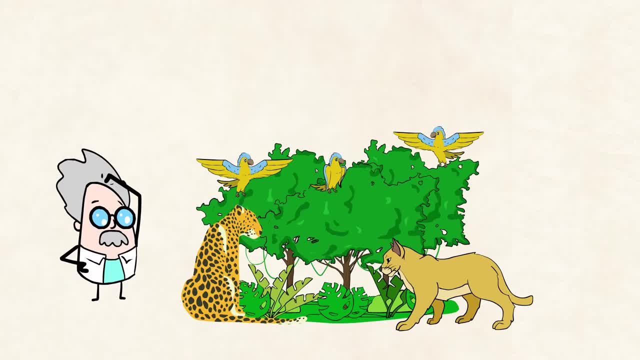 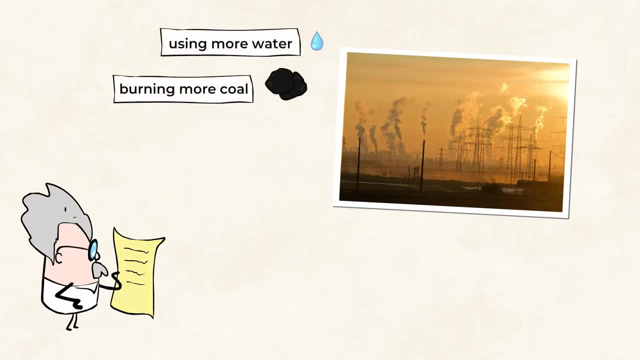 Some adapted, while others moved to find other environments. Some adapted, while others moved to find other environments, And some just couldn't survive. And some just couldn't survive. We also started using more natural resources, such as water, burning more coal and petroleum for fuel. 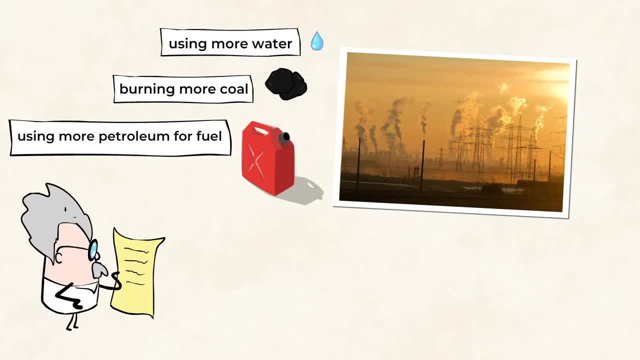 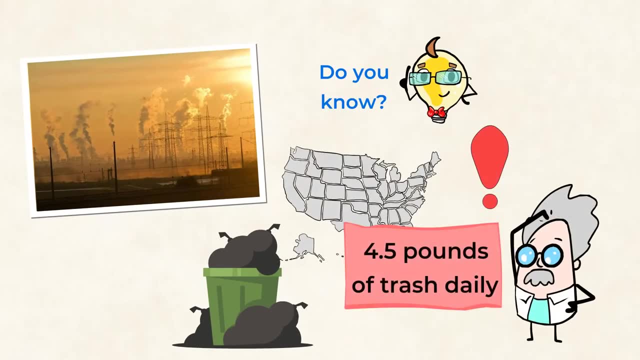 And the more we use them, the more bad chemicals are released and the more garbage is generated. Do you know that a person in the United States creates 4.5 pounds of trash a day? That's an enormous amount- Cars, buses and even cars. 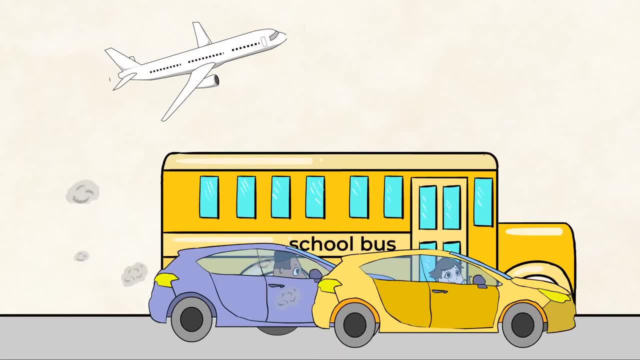 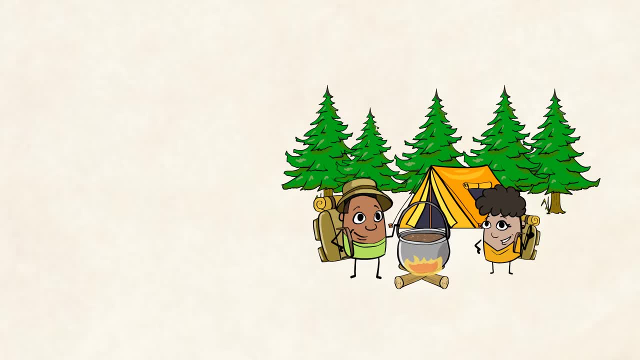 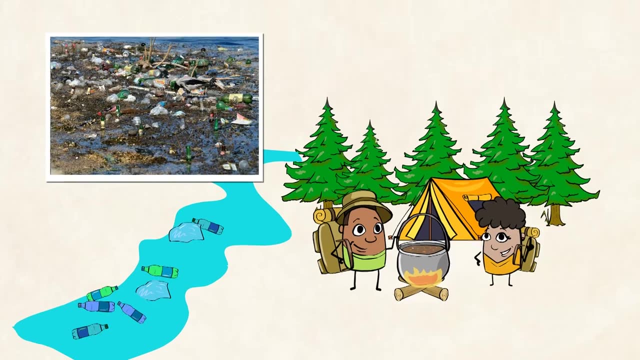 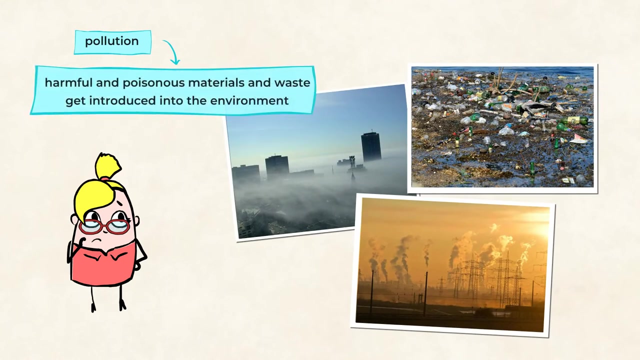 Buses, airplanes and all vehicles generate huge amounts of poisonous gases. Even going camping could lead to fragile vegetation being harmed, And the sometimes left behind waste that ends up floating in waterways can trigger an algae boom. These all cause pollution, as harmful and poisonous materials and waste get introduced into the environment, thus changing it. 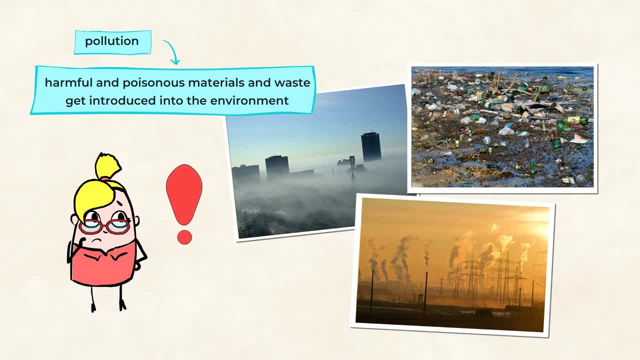 Do you think that pollution is good for plants and animals? Do you think that pollution is good for plants and animals? Do you think that pollution is good for plants and animals, Or even for us humans? Well, if you said no, you're right. 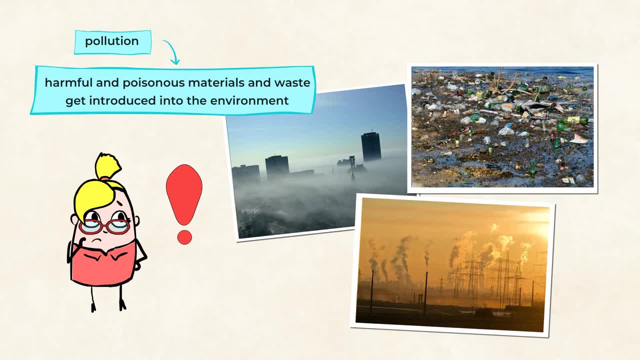 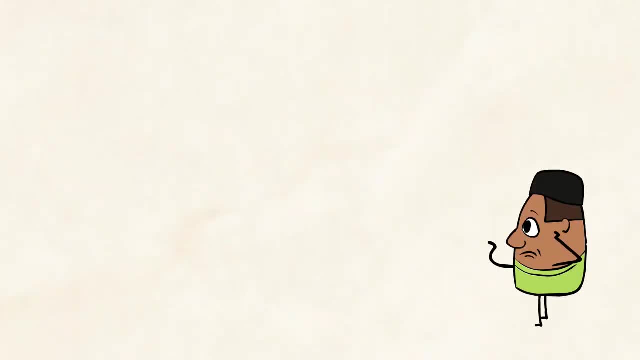 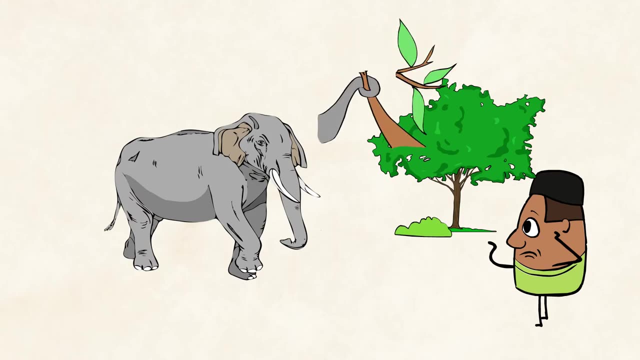 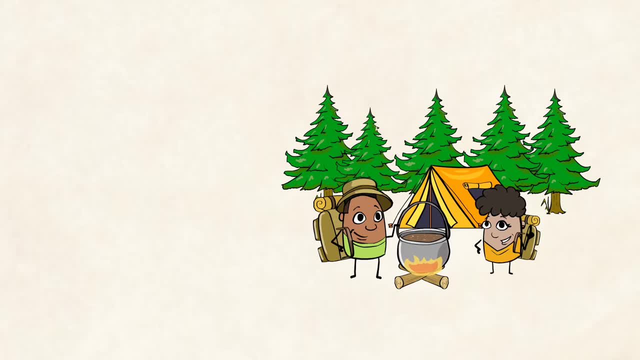 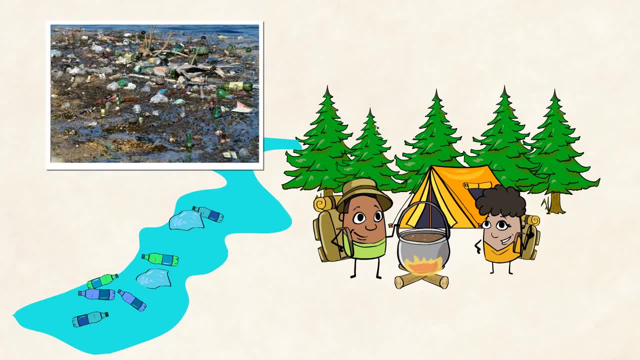 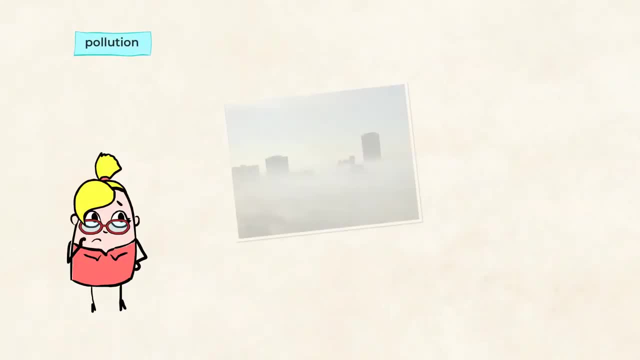 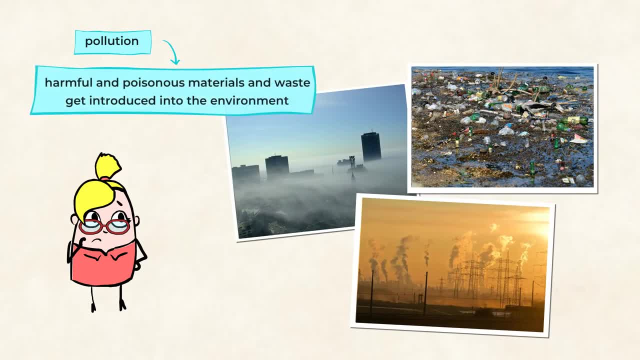 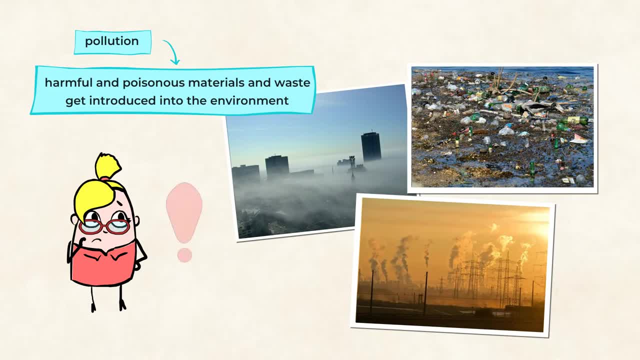 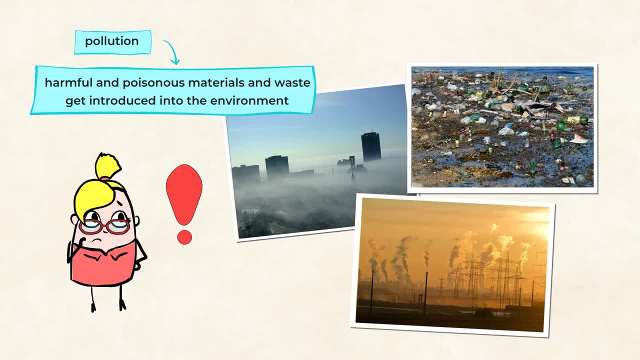 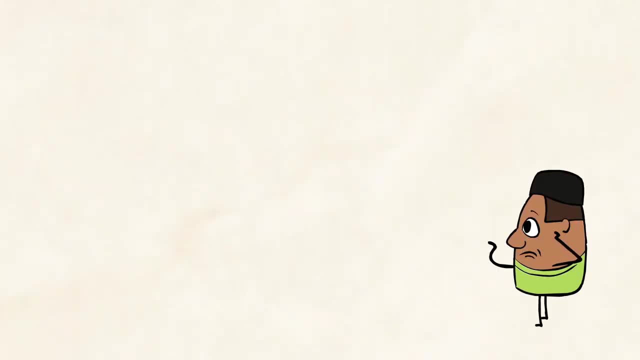 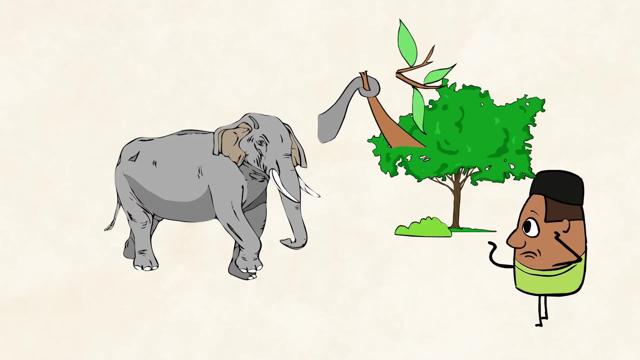 Pollution causes damaging changes to the enviroment. It threatens animals' and plants' ability to survive and their habitats. But it's not just us humans that have an impact on our enviroment. Take, for example, elephants. To reach food, it breaks branches, uproot bushes. 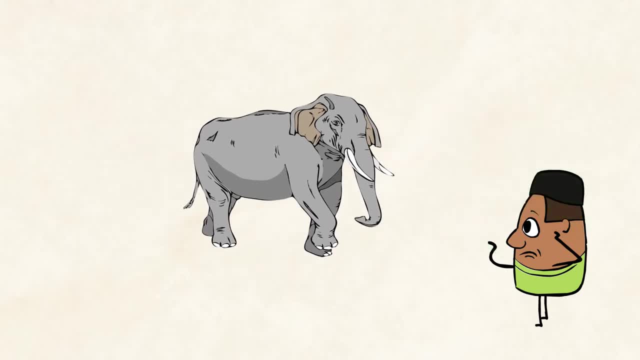 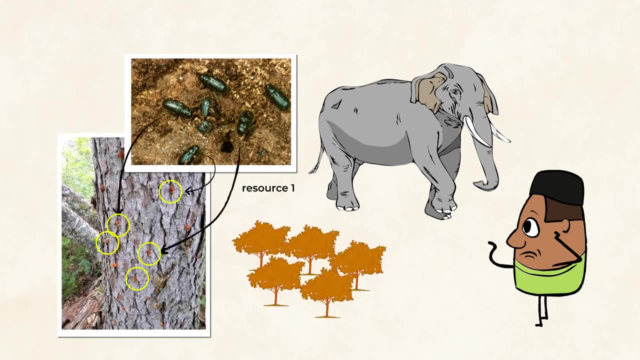 it pushes down trees and bjudga and harm forests, causing environmental changes, And some beetle species are known to kill live trees. Whole forests can even be destroyed if they get out of control, And beavers also cause major change to the environment. 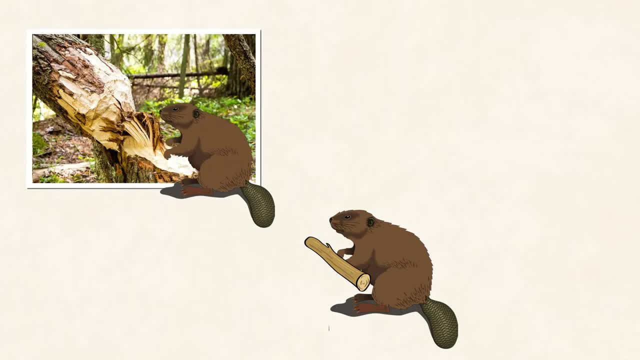 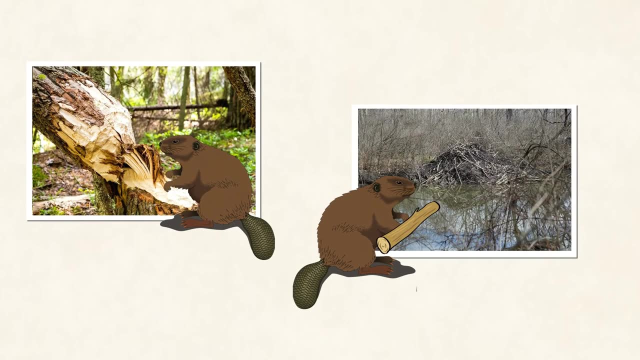 They eat on trees And it takes just about five minutes for a beaver to cut down a whole tree. Now they use some part of the tree to build dams and rivers, which create an entirely new habitat, changing the environment around them. 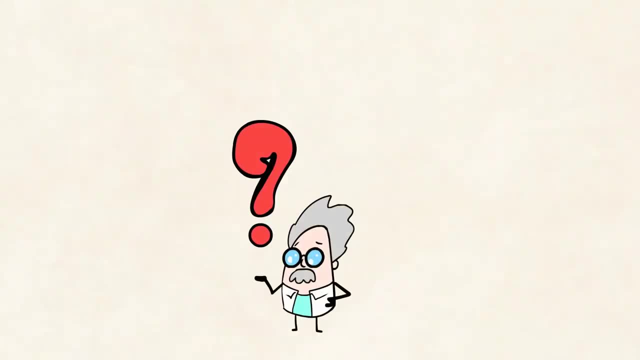 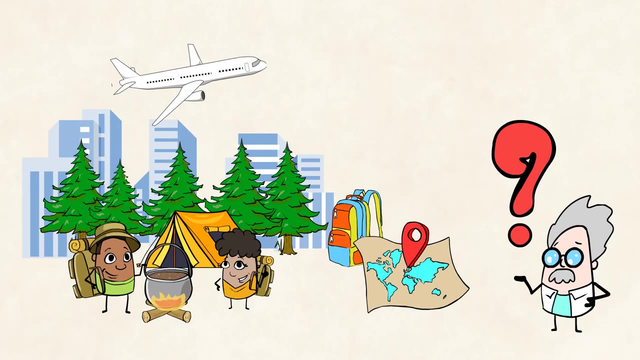 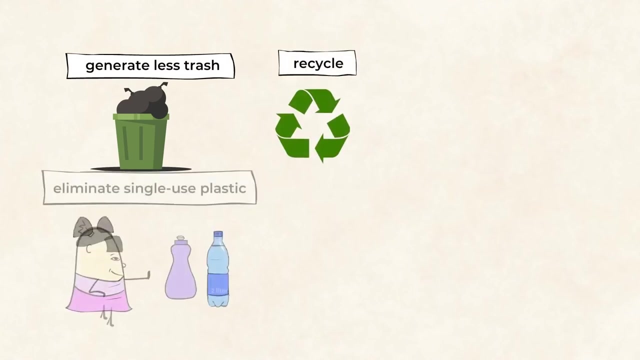 So what can we do to preserve our environment and change it for the better? We can't stop traveling, exploring, building, Nor can we change nature, But we can do simple things like generate less trash, recycle more, eliminate single-use plastic, take showers instead of baths. 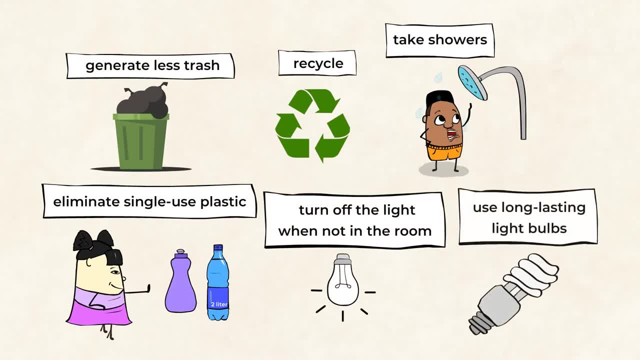 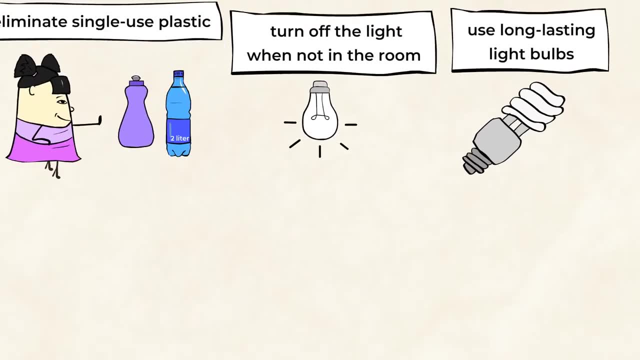 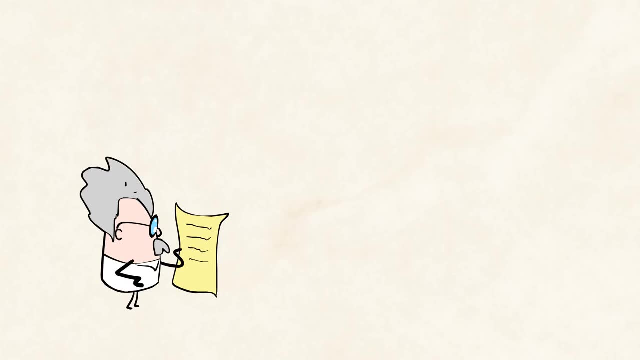 turn off the light when not in the room and use long-lasting lightbulbs. You have no idea how much these little things will end up helping the environment. Scientists are constantly looking into various ways to reduce pollution, coming up with solutions to reduce our consumption of fuel.